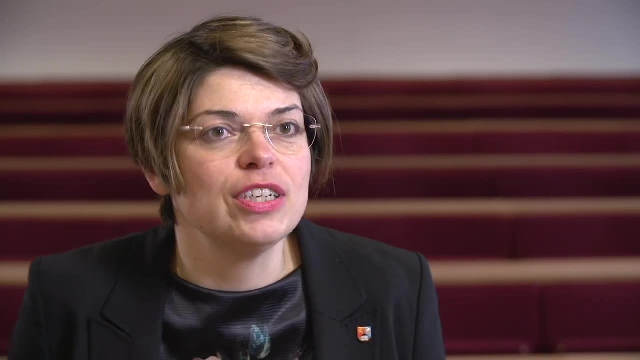 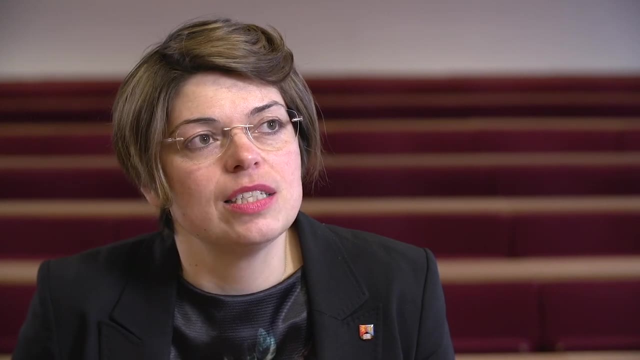 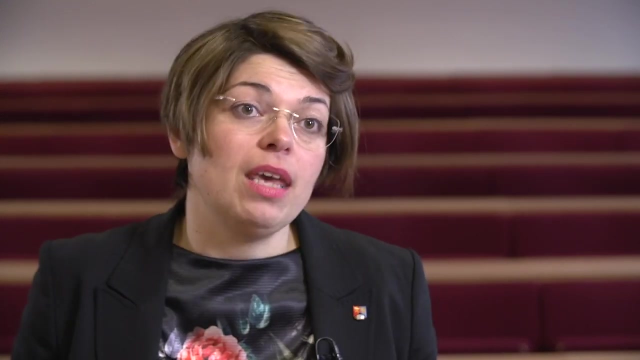 in the whole of the UK, So that, as a first, is already rather unique. What I can say is very unique in terms of the teaching and the experience you gonna get if you come to study with us and do this program is that you will get me and all the people around me, All our 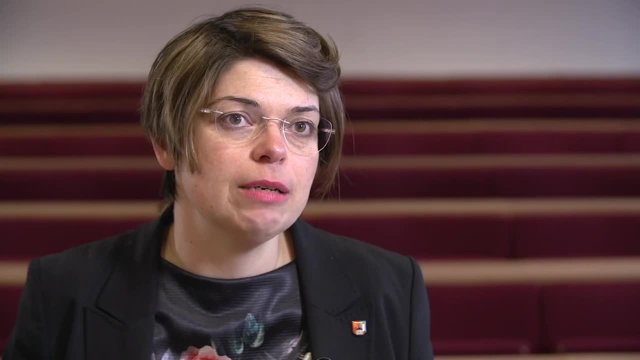 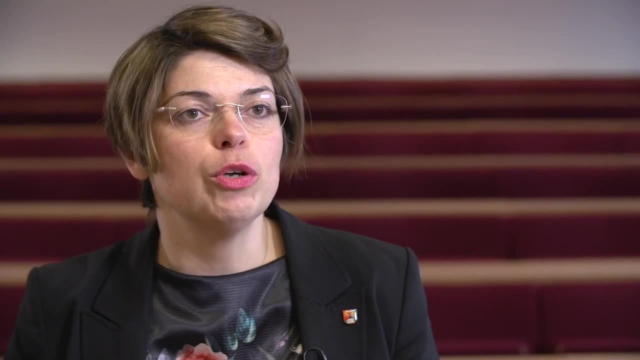 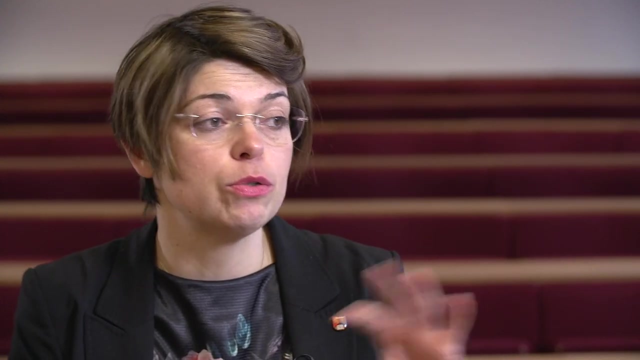 excellent experts, researchers, who are doing the teaching, but also we take on board a lot of the industry companies. so what we have on the program is we have an industrial advisory board. so we have members of the big, and not only the big, also of the smaller companies within the 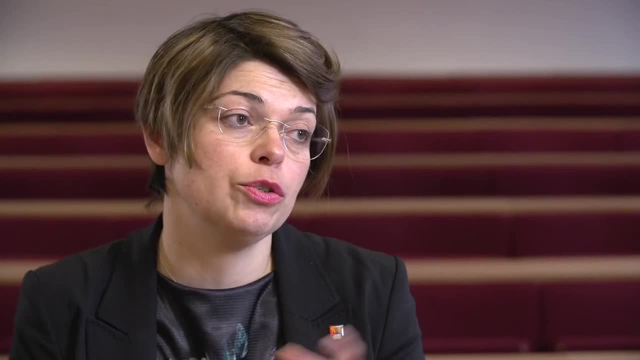 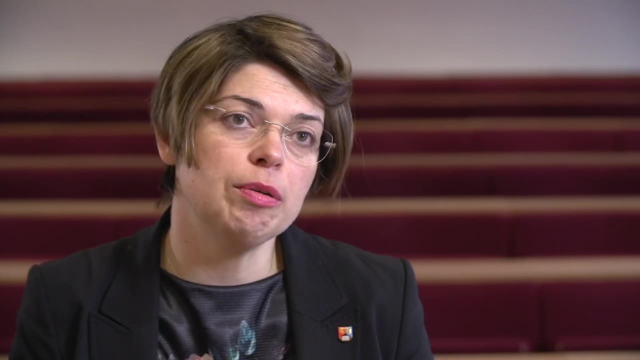 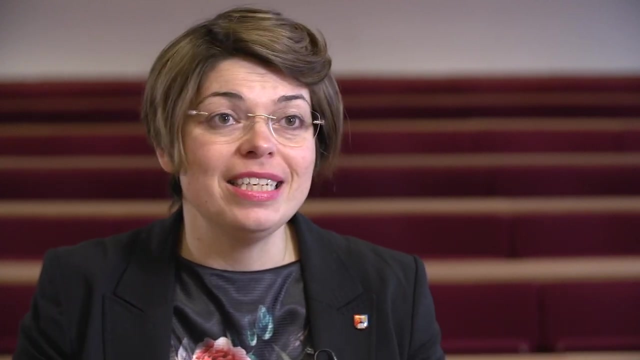 UK companies which are connected or do work on nuclear decommissioning and vice management and they meet with me twice a year where we discuss the program. we discuss if the needs of the industry require a little bit of change in our syllabus, depending on what the needs of the market are, you know. so we are trying. 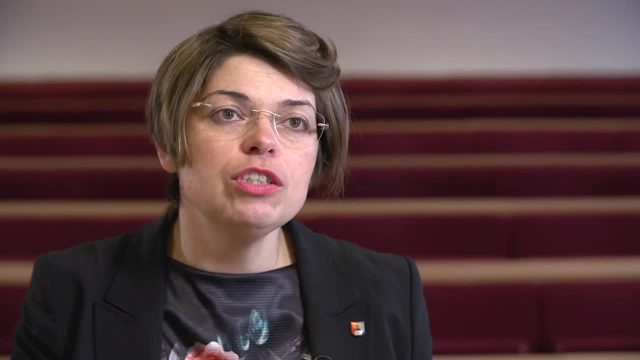 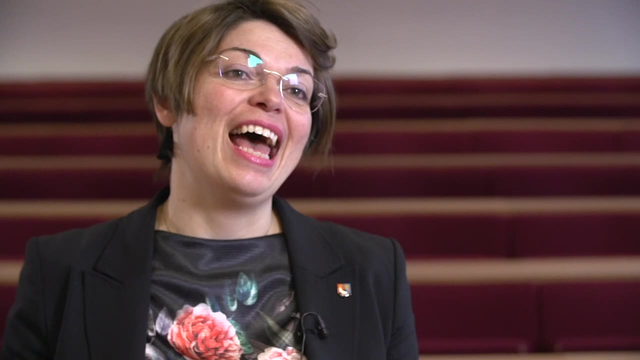 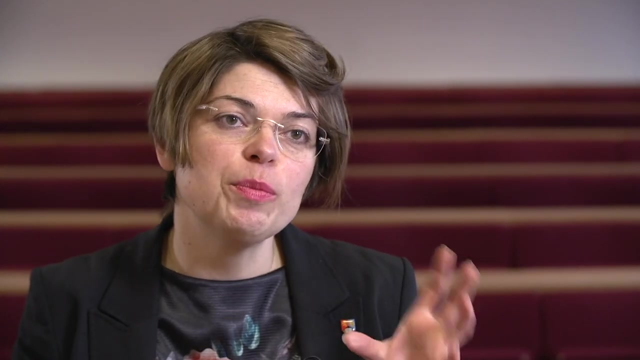 to really tailor the syllabus and the knowledge of our students to what the needs of the industry are. we're also very friendly and I do look after my students on a personal basis. if you come to us, you'll be really considered as a person, not as a number. 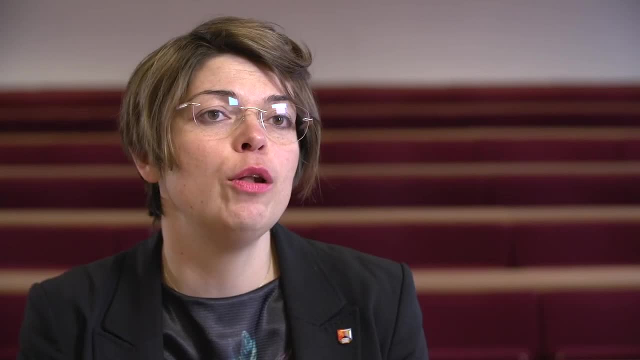 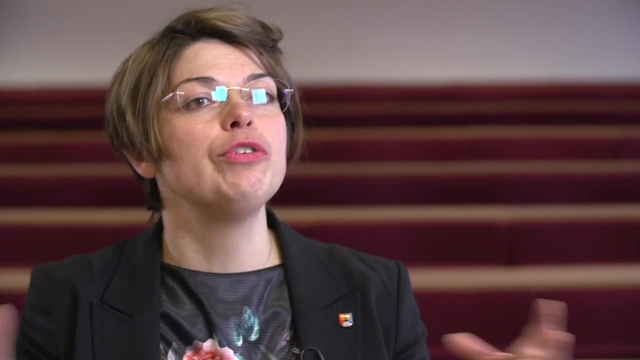 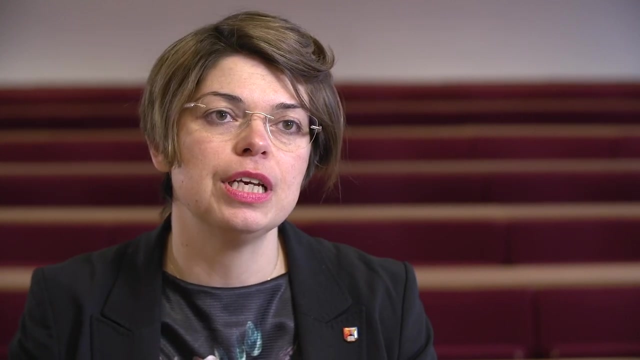 and you'll be really individually looked after. I really take care that I take into account what your skills are, what your wishes are, and we try to during that whole year of education. I also try to mentor a little bit the students in direction. that's what they wanted when they come. that's what they want now. 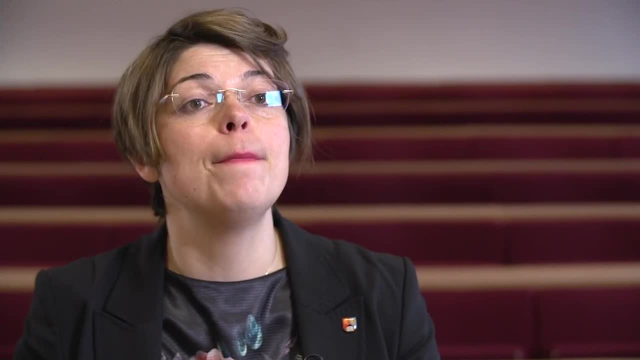 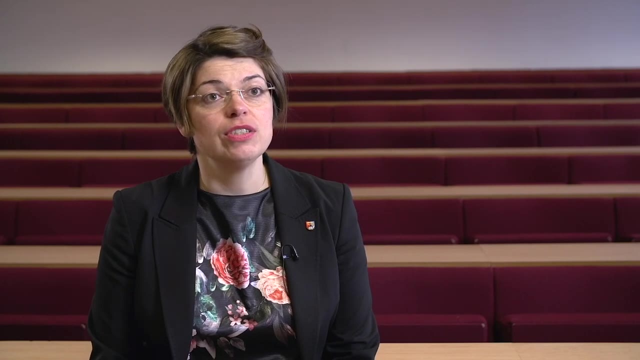 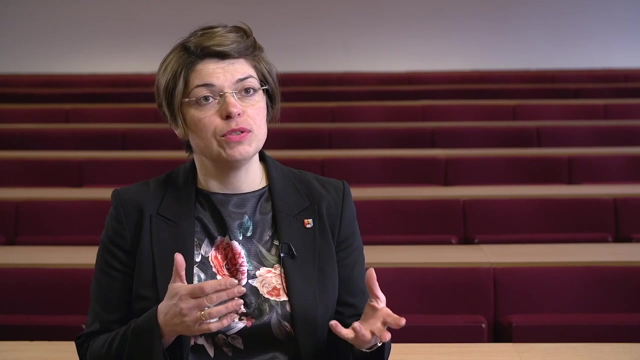 that's the set of skills they have. how can we work best to their strengths so they'll get the best job afterwards? our program is aimed at postgraduate, so people who are looking into career in the nuclear industry, and they can be at various levels of their study in terms. 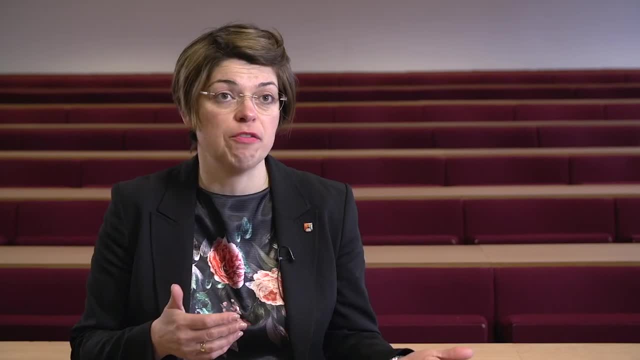 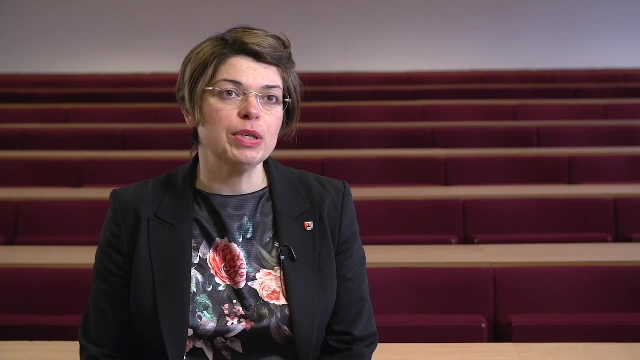 of that. they could be in the third year looking to what they're going to do after they finish their BSc, or they could be also mastery students who are just looking for alternative for their fourth year. so in principle, we take students after their bachelors, after they have two, two or higher great and 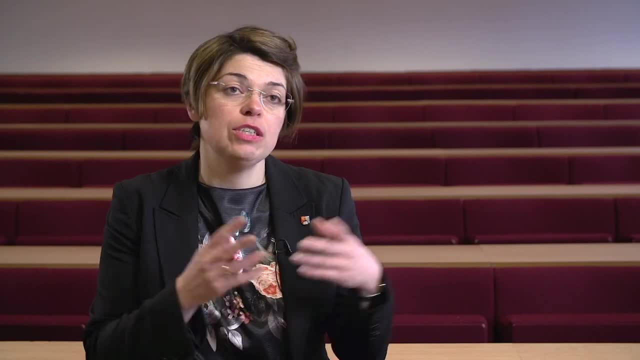 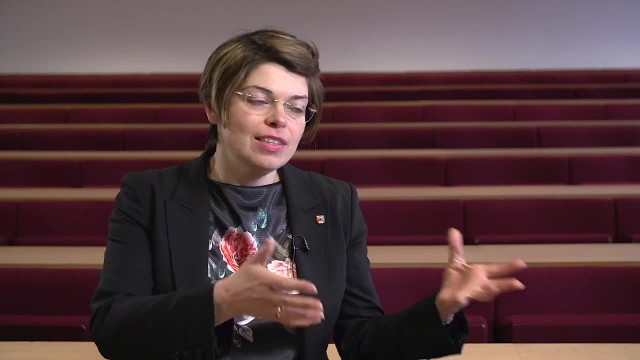 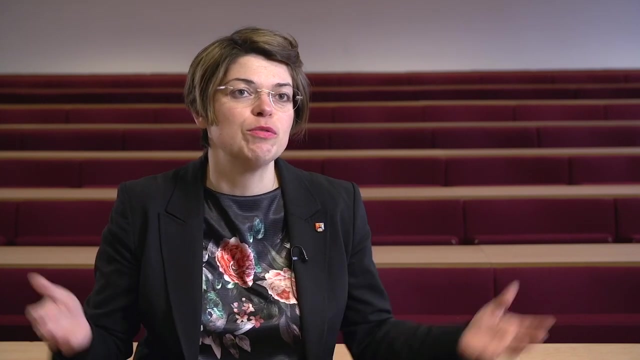 also we take some people who have finished their study, took a break or worked for some time in the industry somewhere else and decided they want to change their career and start. you know, take some other degree which will help them to find a secure job and also be involved in the nuclear industry. what you need to 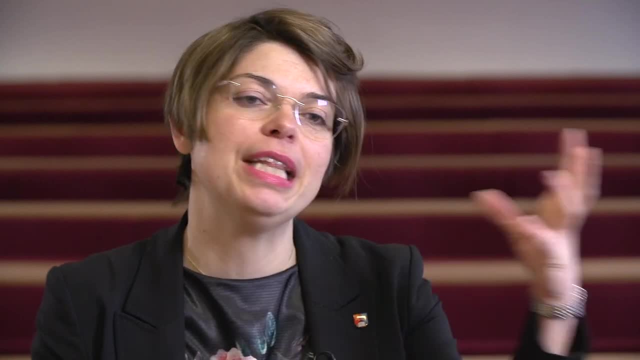 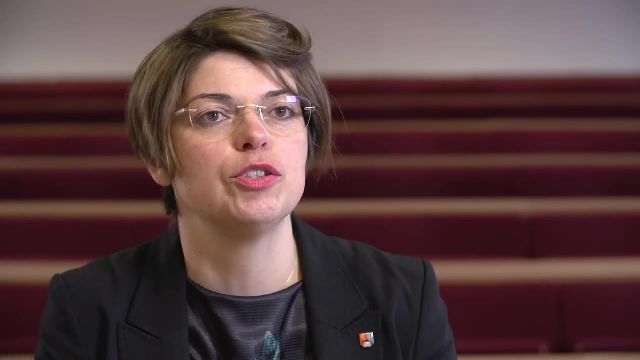 know about the program in terms of coming here so you can read. all the details are online on our internet page. you can see exactly what type of modules we have, with little descriptions and it's actually so. things you need to know when you're coming here as a student are: 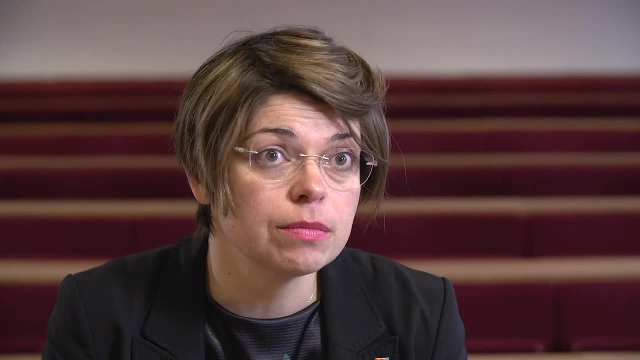 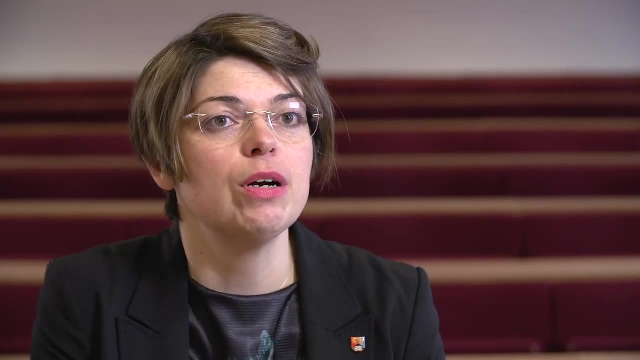 probably the following: it's going to be not an easy year. it's a hundred twenty credits, so you have to earn them, you know. so you're not going to get any presents there, because we have to prepare you for what is expecting afterwards. we are highly respected. 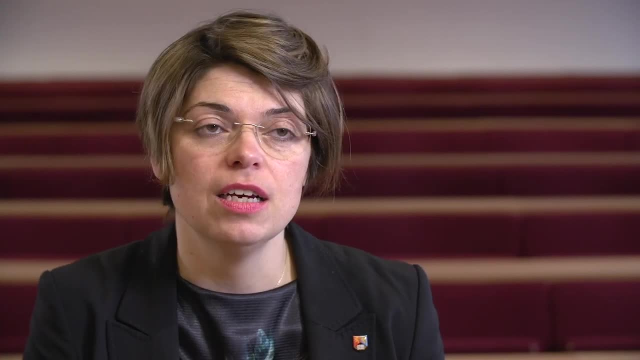 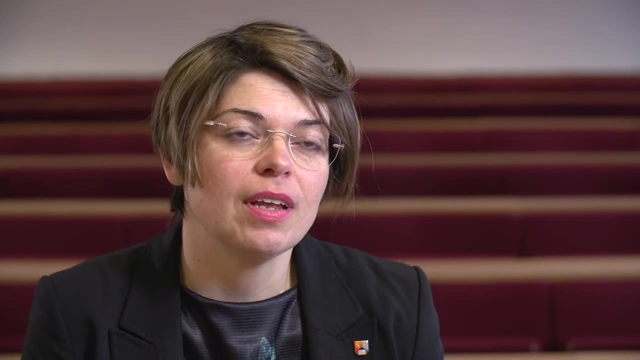 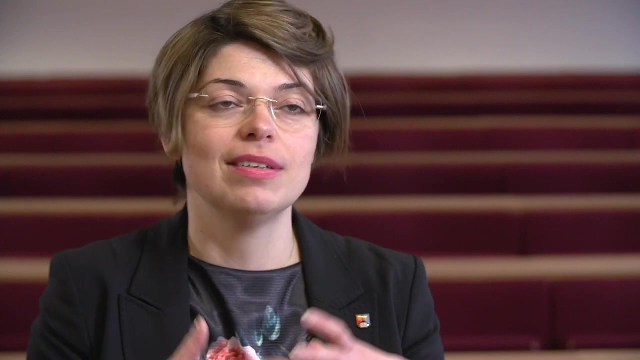 university, the school of physics and astronomy. it has a great reputation, but we have it only because we work hard and we deliver. so if you want to work hard, you'll have all the opportunities to get the grades you're coming for. so we help you, but also, what we do is we. 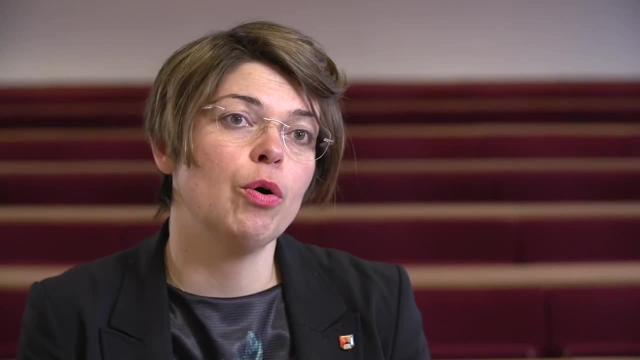 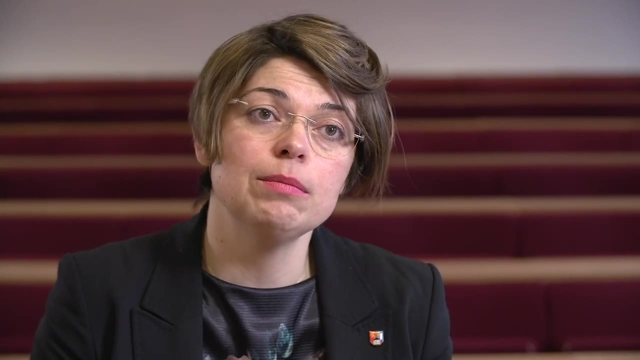 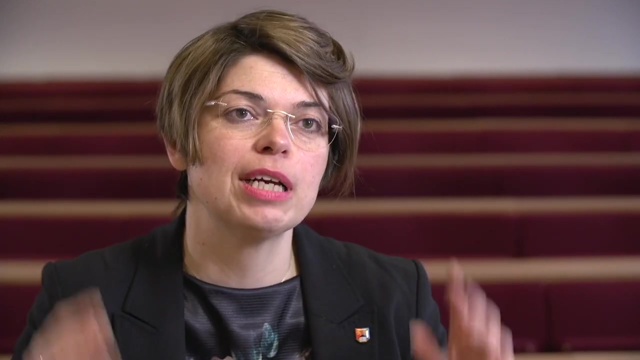 have something called canvas which helps us record all the lectures, of all our lectures, and this will give you the opportunity, in your own time, in your own pace, to also go through the lectures again and again until you really have the eureka momentum. no, so, until you really find out what, what you need to, to 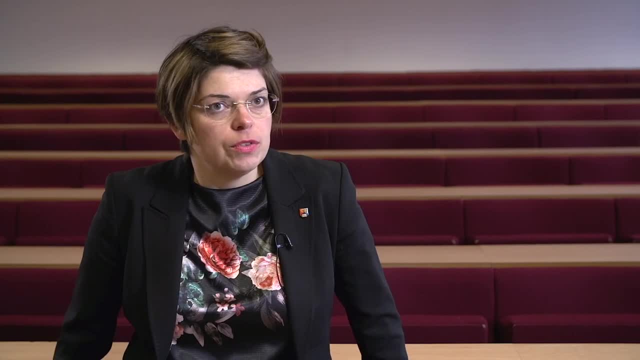 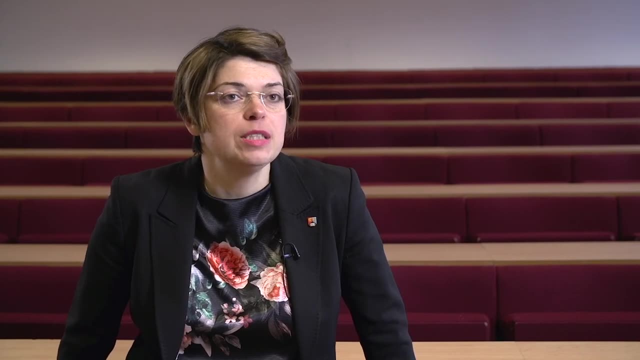 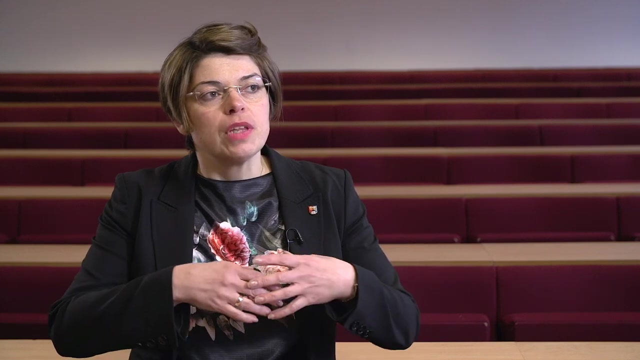 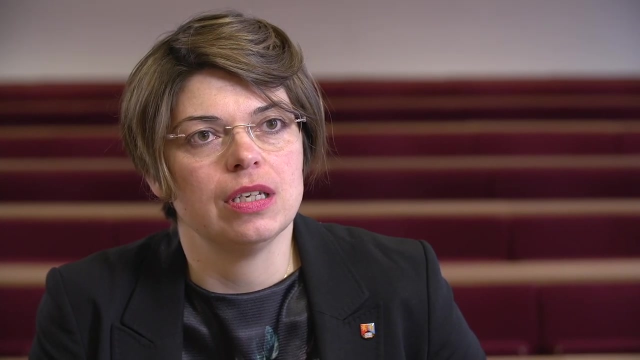 do the aims of the program in terms of career outcomes. so the program is aimed really at diverse students at from diverse backgrounds. since nuclear, the commissioning and waste management is also an area which bridges between a lot of different areas of expertise, one of the other points which is strong in terms of what we do here in Birmingham. 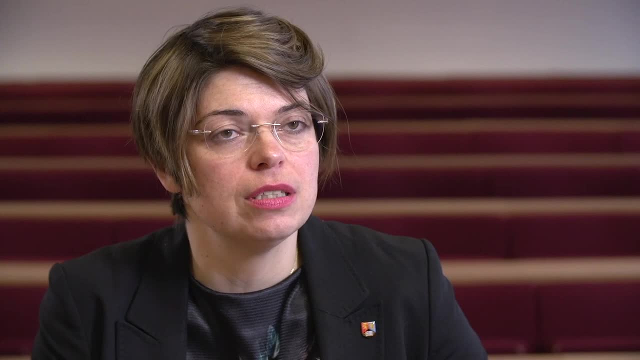 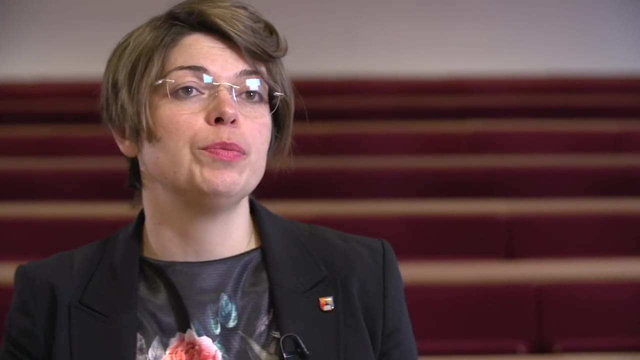 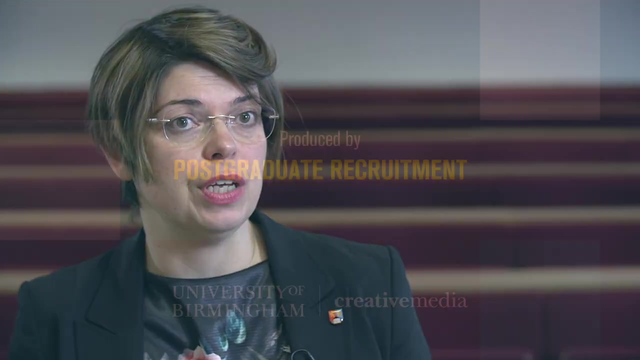 in terms in direction of nuclear education is is those strong connections we have with the industrial partners. so, as I mentioned before, this gives us an opportunity to shape the program and the syllabus, but it also gives us some flexibility when it comes to funding.